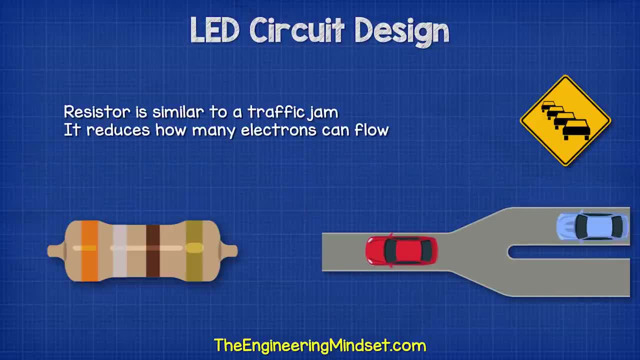 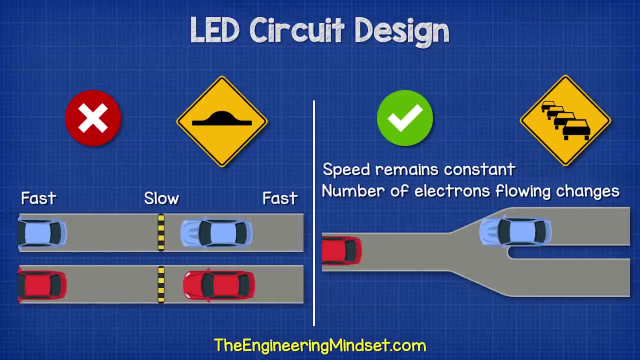 will flow in this simple series circuit. The resistor acts something like a traffic jam, reducing how many electrons can flow. Most people incorrectly assume it acts like a speed bump and that the electrons must be slowing down just before the resistor and then speeding up again. 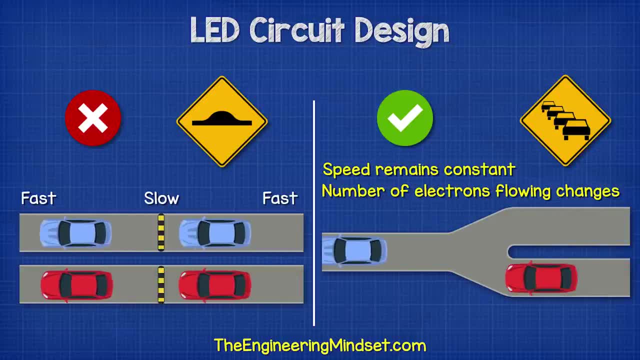 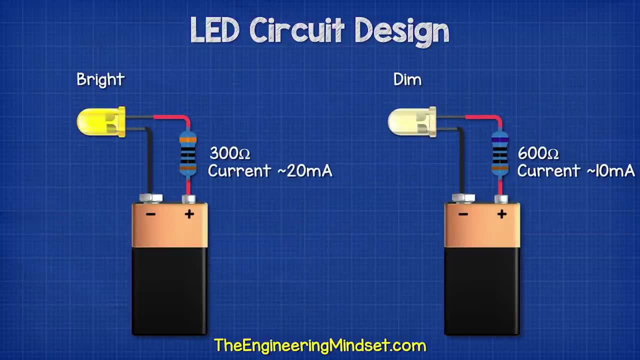 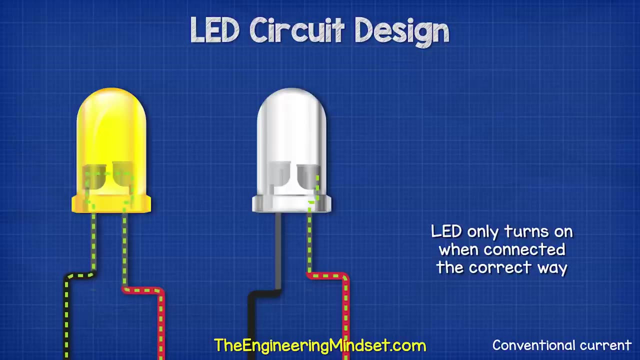 The speed of the electrons remains constant. The number of electrons flowing is what changes. The higher the resistor value used, the lower the current will be, and so the dimmer the LED will shine. We need to remember that LEDs will only allow current to flow in one direction. 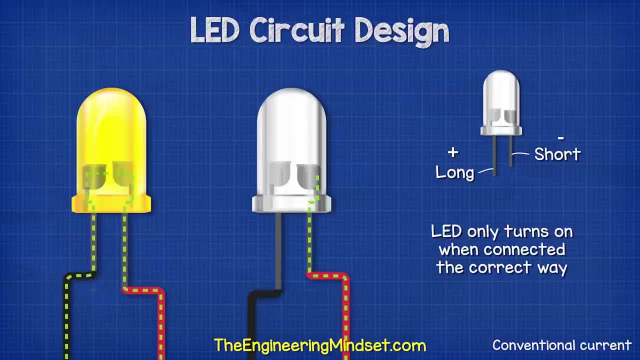 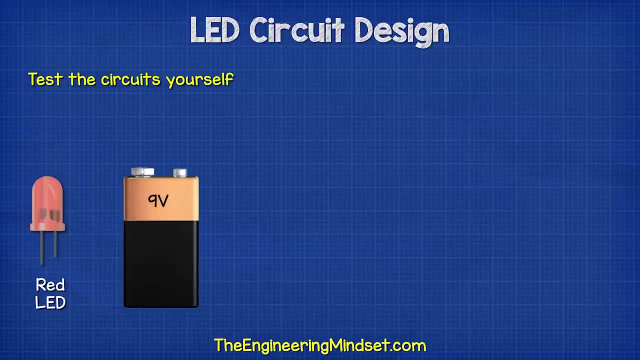 with the positive connected to the long lead and the negative connected to the short lead. If we connect the LED the other way around, it will simply block the current and the LED will not turn on. You can test this circuit yourself. Take a red LED, a 9V battery, a resistor of between 360 and 390 ohms, another higher 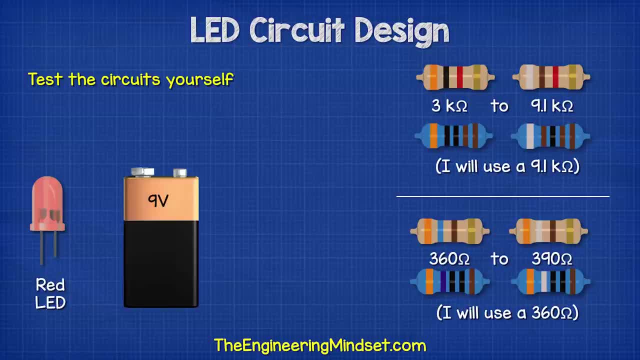 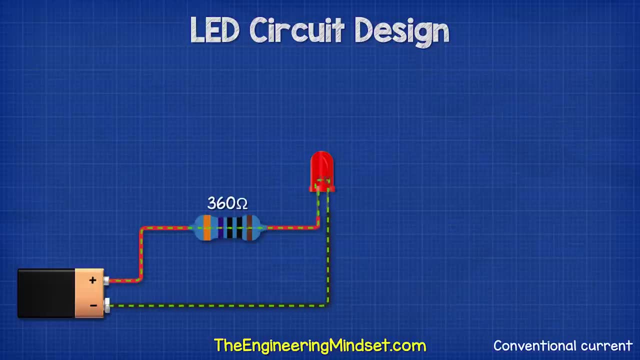 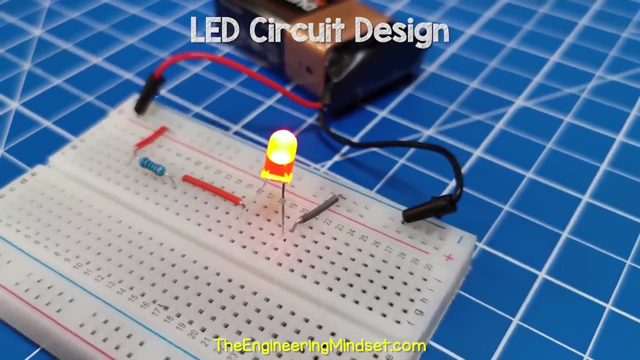 value resistor of between 3k ohms and 9.1k ohms and a multimeter. Connect the low value resistor and the LED to the battery in series and the LED will illuminate. I am using a breadboard for this, which makes it very quick and easy to test electrical circuits, but 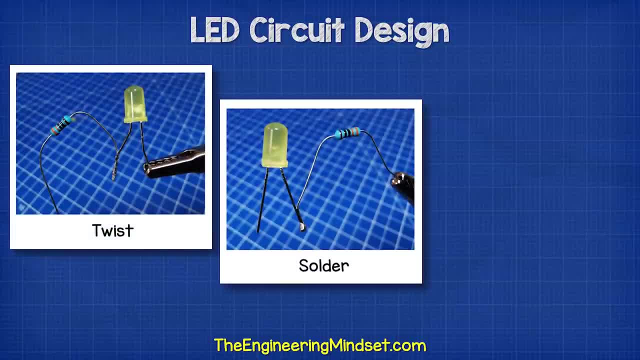 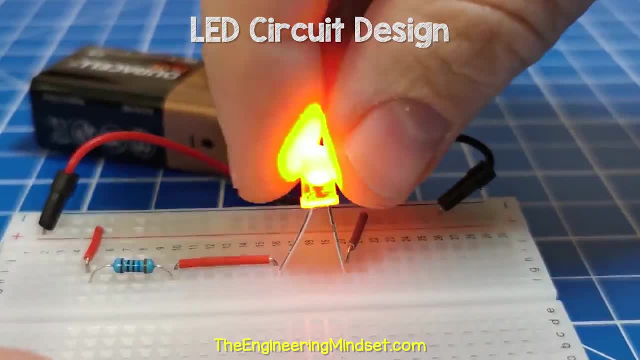 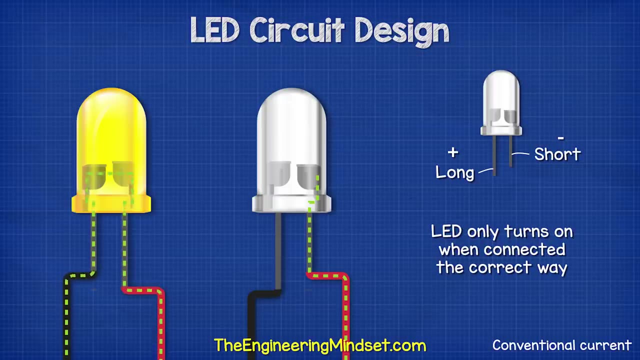 you can also just twist the wires together, You could solder them or you can use some connectors and it will all work fine for this simple experiment. Notice that if we turn the LED around, we see it blocks the current, so it will not illuminate. It only works in one direction. 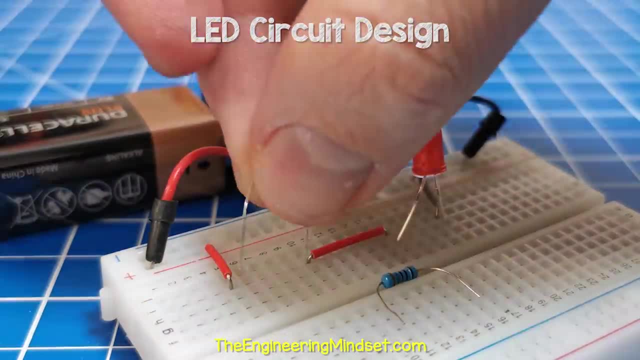 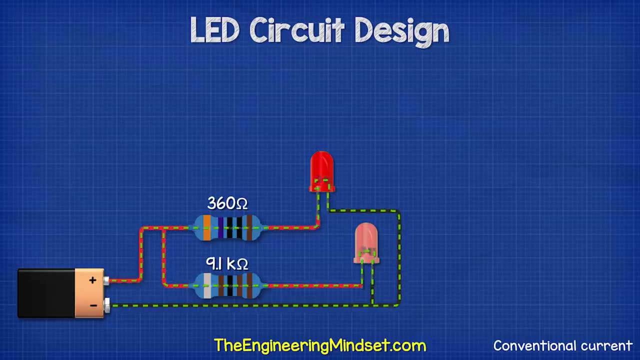 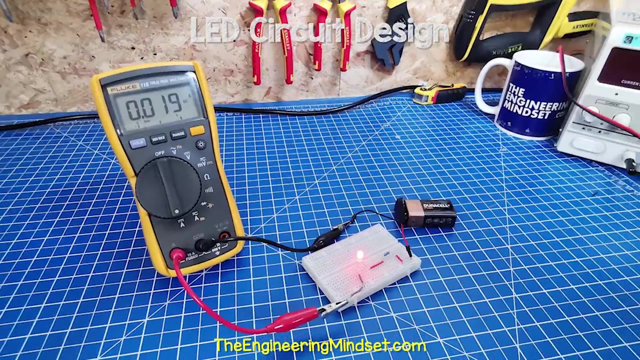 If we replace the resistor with the high value 9.1k ohm resistor, we see the LED is very dim. We can also connect them in parallel to compare the brightness. So now with the 360 ohm resistor and the LED in series, we can connect our multimeter into. 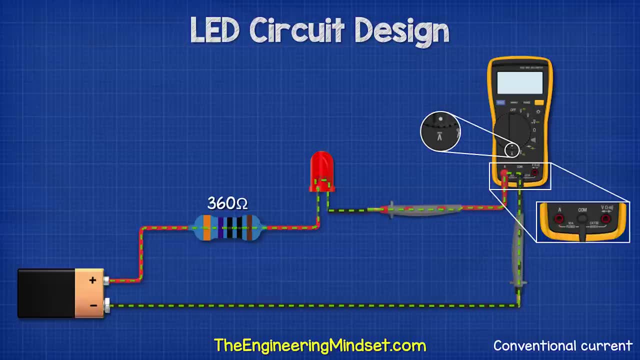 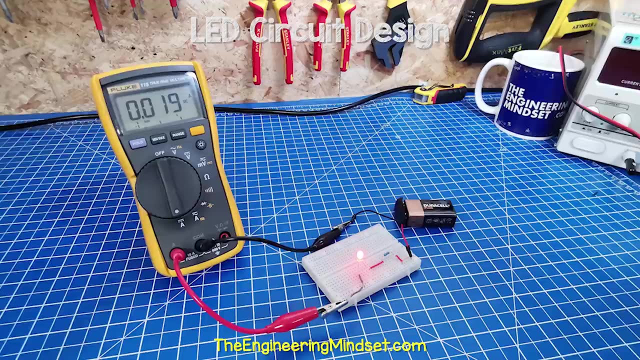 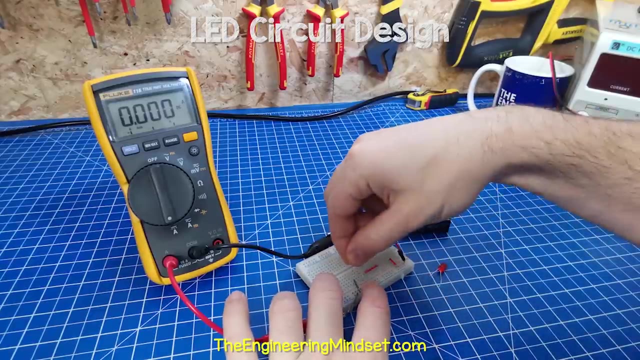 the circuit, making sure to place the multimeter into the current reading mode. We should see somewhere between 17 and 20 mA, depending on which LED and resistor you've used. We can switch the position of the LED and the resistor. It will work fine and give us the same current reading. 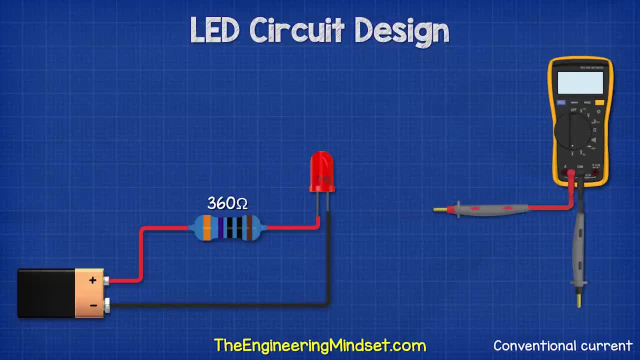 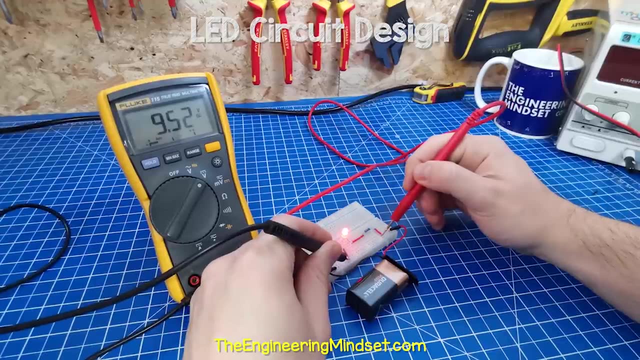 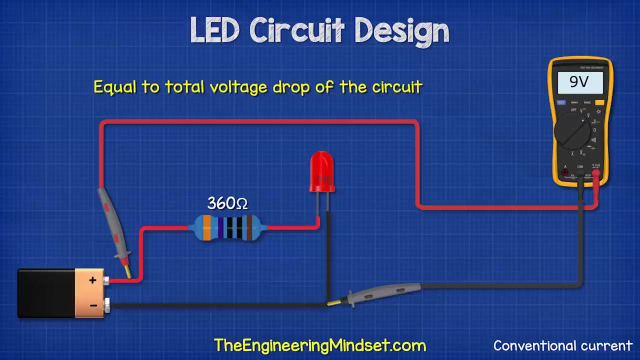 Now remove the multimeter from the circuit and place the multimeter into the DC voltage mode, Measure across the two far ends of the circuit and we should see around 9 volts. This is what the battery is providing to our circuit and it is also equal to the total voltage drop of the circuit. 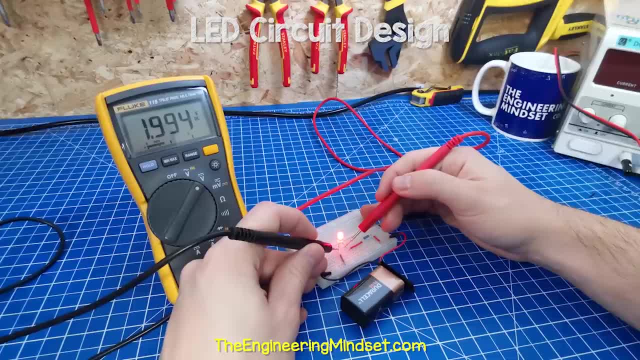 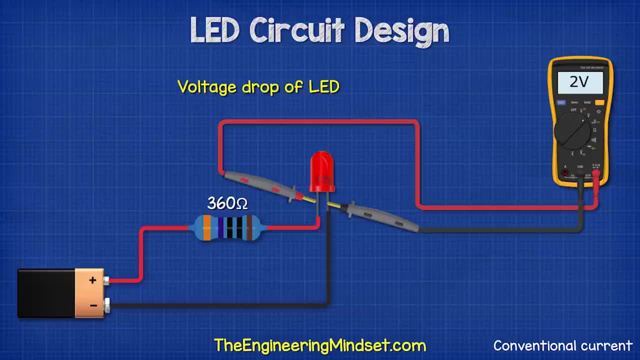 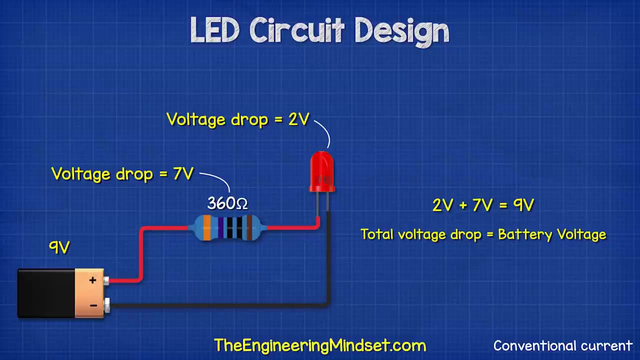 Now measure across the LED and we should see around 2 volts. This is the voltage drop of the LED. It's removing two volts from our circuit. Now measure across the resistor and we should see a voltage drop for the remaining seven volts. So two volts plus seven volts is nine volts, which is the same. 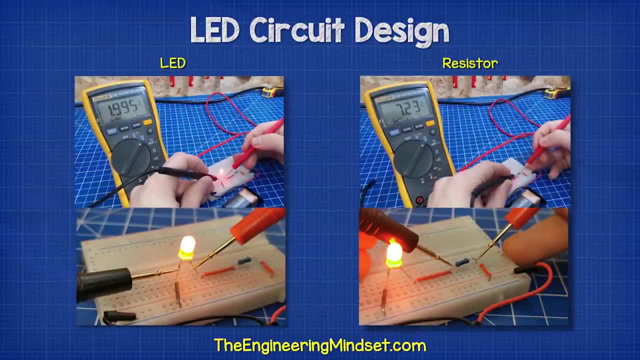 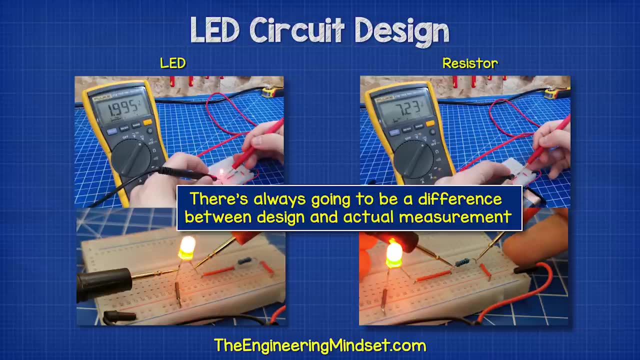 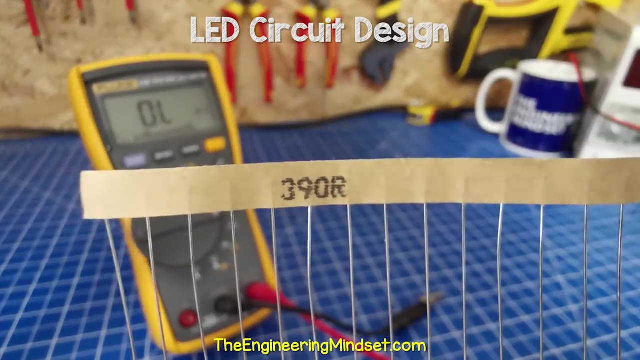 as our battery. You might have noticed that the values measured weren't exactly two volts, seven volts or even nine volts. There's always going to be a difference between the design and the actual measurement. For example, this resistor is rated for 390 ohms, but when we measure it it's actually 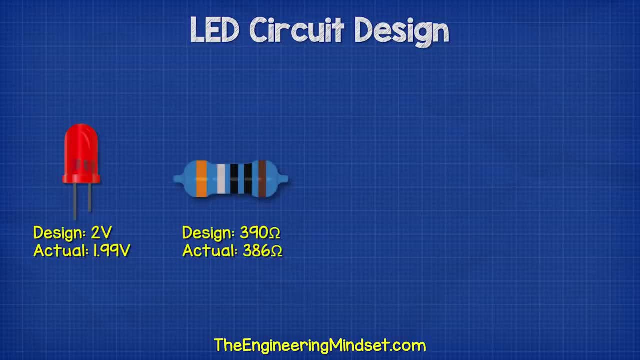 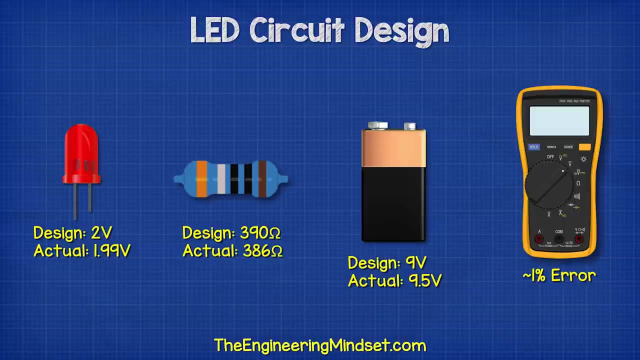 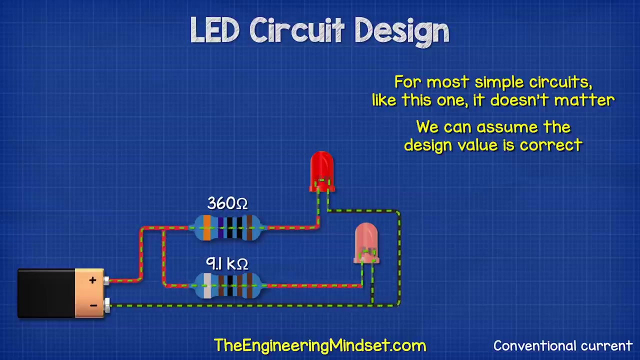 386 ohms. Each component, including your multimeter, will have an error tolerance. It will be close to the design value, but never exactly this value. For most circuits like these simple ones, it doesn't matter. We can assume the design values are correct, Just remember. 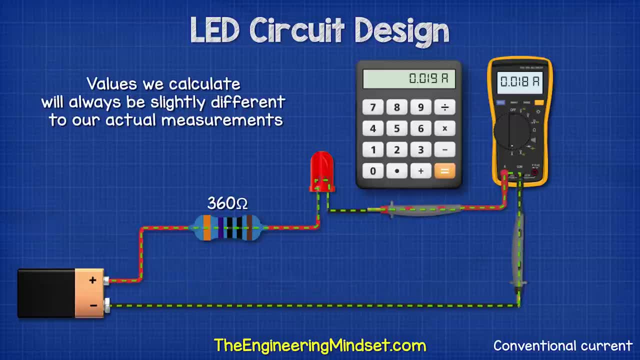 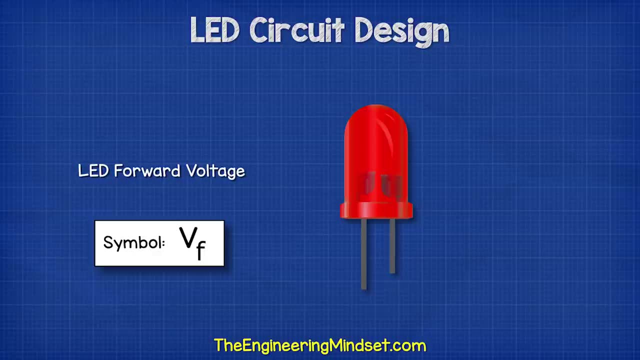 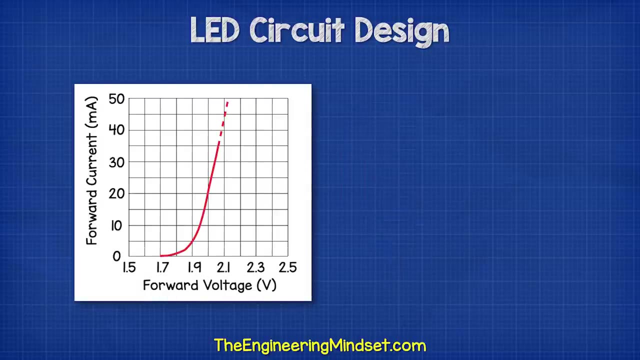 that the design values are correct, That the values we calculate will always be slightly different to our actual measurements. We also need to know about the forward voltage. This is basically just the voltage drop we measured earlier. The manufacturer will provide a chart like this one, which shows the forward. 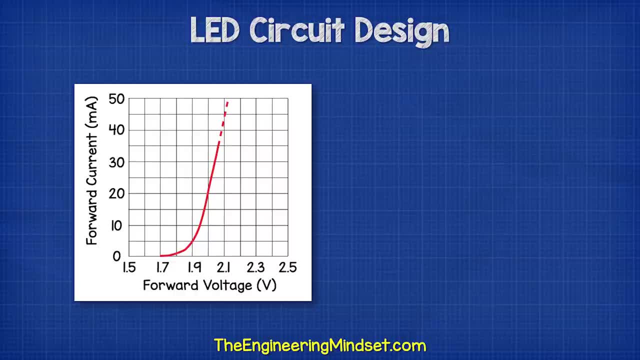 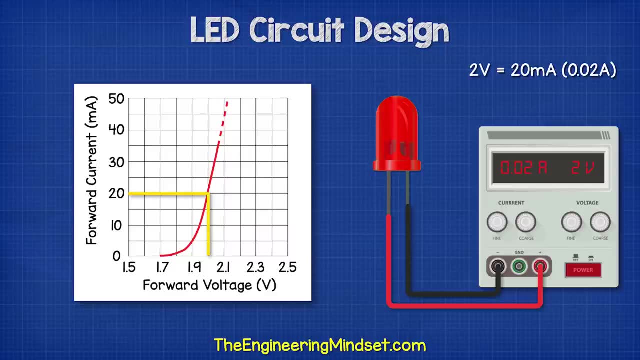 current at a given forward voltage. So if we connect a voltage source across the leads and apply two volts, we should see 20 milliamps of current flowing. If we supplied 1.6 volts, we should see 0 milliamps, because the LED will be off The chart for this. 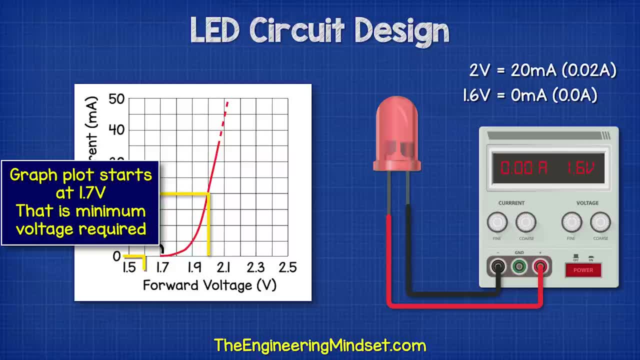 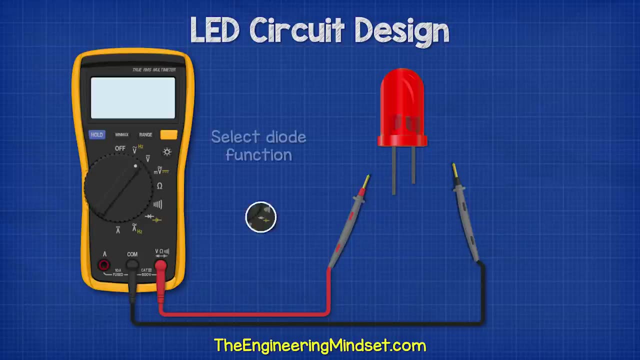 LED begins at around 1.7 volts, So we know that we need to provide a minimum of 1.7 volts for this LED to start illuminating. We can test our LED's minimum opening voltage using a multimeter. If you select the diode mode on your multimeter and then connect the red lead to the multimeter, you can. 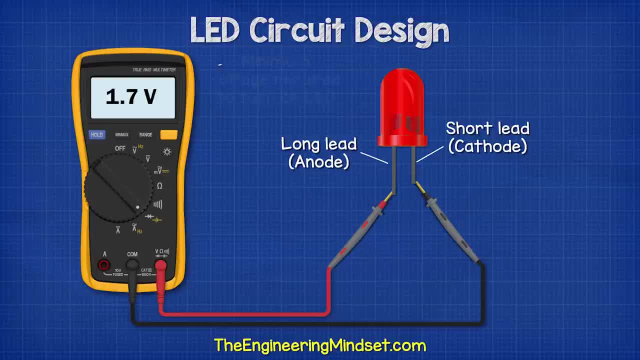 see the LED lines there. By connecting the red led to the long anode and then the black lead to the short cathode of a red LED, we should see something like 1.7 volts. so this is the minimum voltage required to turn the LED on. 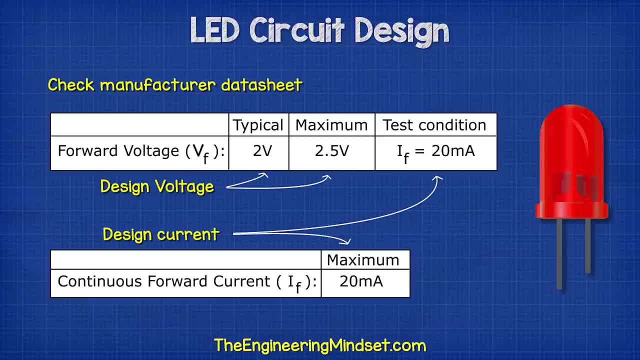 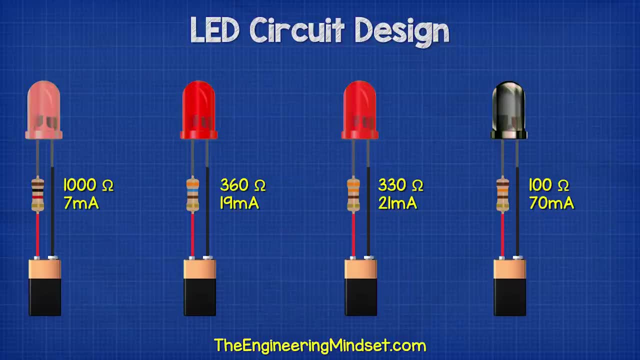 Most standard LED's are rated for a current of 20 milliamps or 0.02 amps. We want to try and stick to this value. If we go below this, then the LED will be dim. if we go too far above this, then the 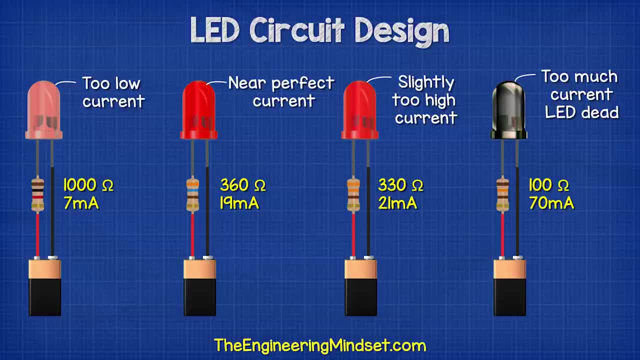 LED will fade itself out. This coil chain will be tin oroncé of 10 milliamperes of energy. If the home厨 LED will be destroyed, We can go above 20 milliamps, but the lifespan of the LED will reduce the higher. 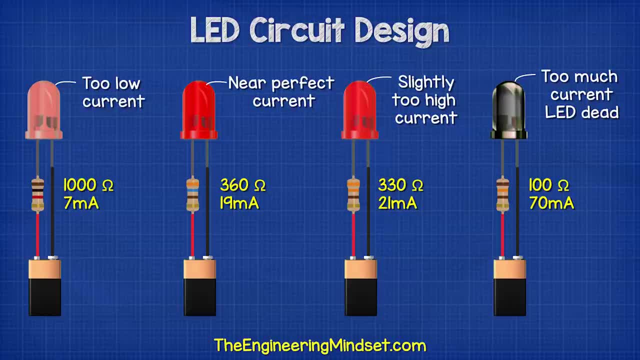 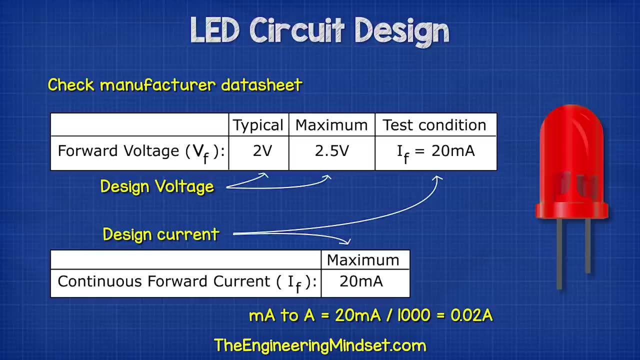 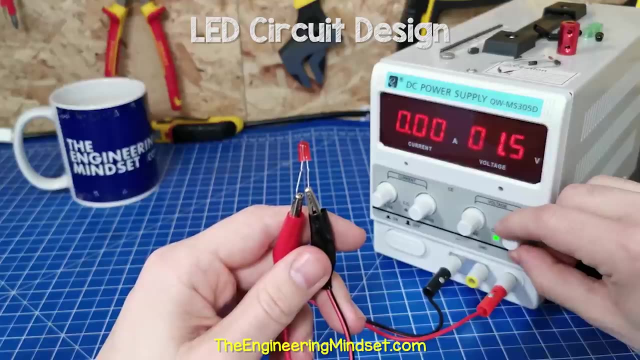 we go. We'll see how to calculate that a little later in the video. The red LED typically has a voltage drop or forward voltage of 2 volts and this will result in a 20 milliamps of current in our circuit. We can test that with a DC power supply When I set the voltage at a constant 2. 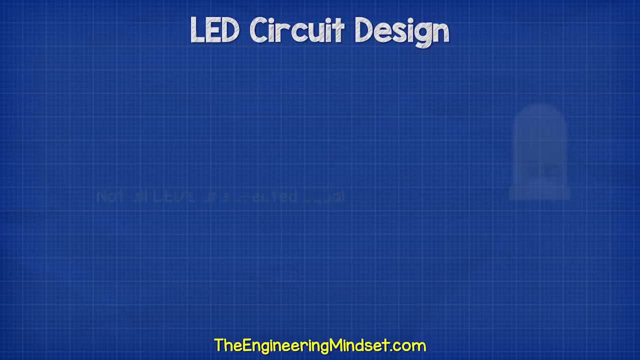 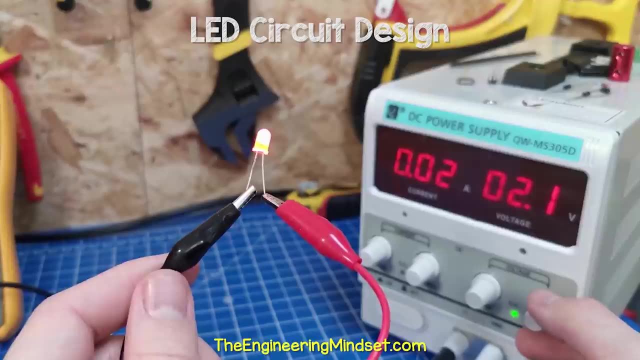 volts, we see 20 milliamps of current, but not all LEDs are created equally. This one doesn't reach 20 milliamps until 2.1 volts are supplied, and this one doesn't reach 20 milliamps until 3.7. 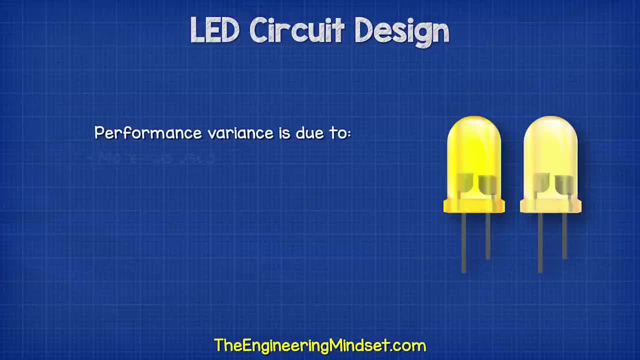 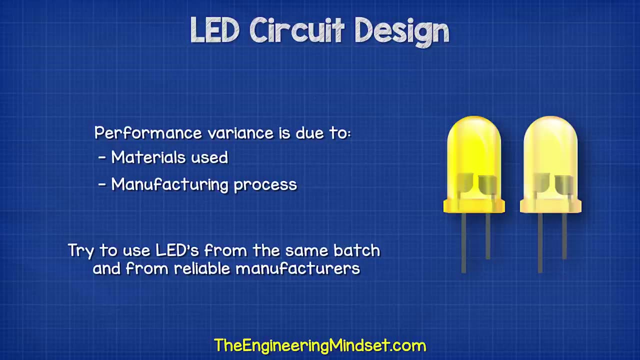 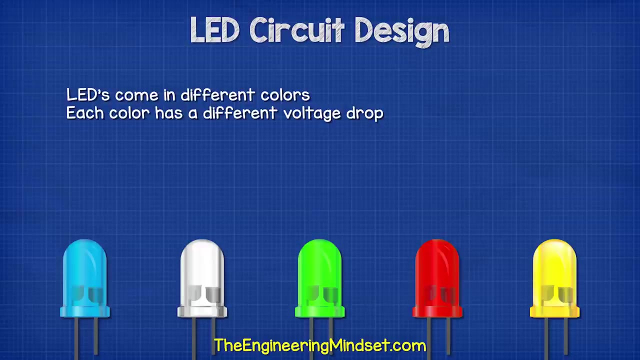 volts is applied. This variance is due to the materials used and also the manufacturing process undertaken, So you should always try to use LEDs from the same batch and also from reliable manufacturers. LEDs also come in many different colors and each color has a different voltage drop also. 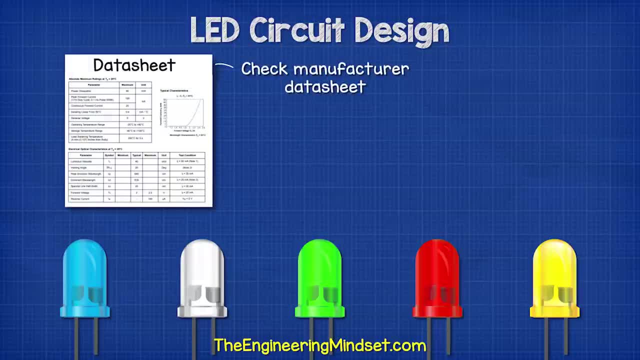 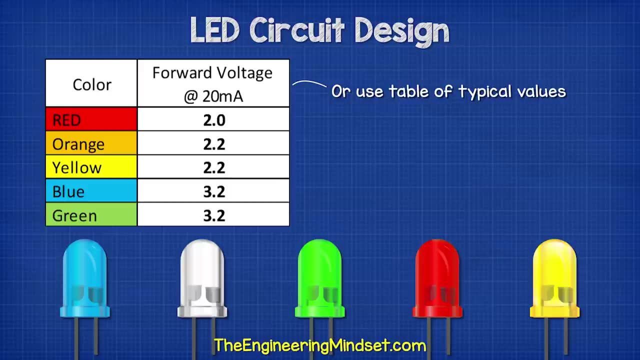 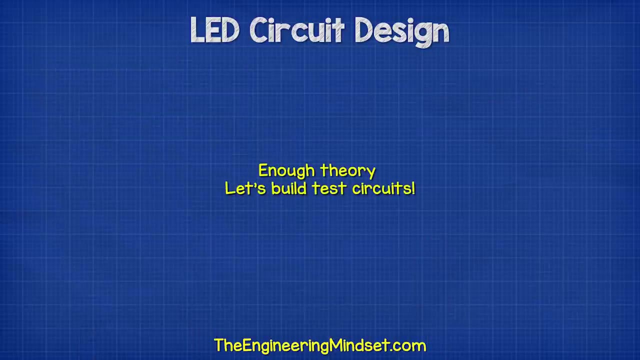 So you will need to look these values up from the manufacturer's data, or you can also test them yourself, or you can use these typical values from these standard charts, but they might not match the LED you actually have. Okay, that's the basics covered, so let's move on and make some example. 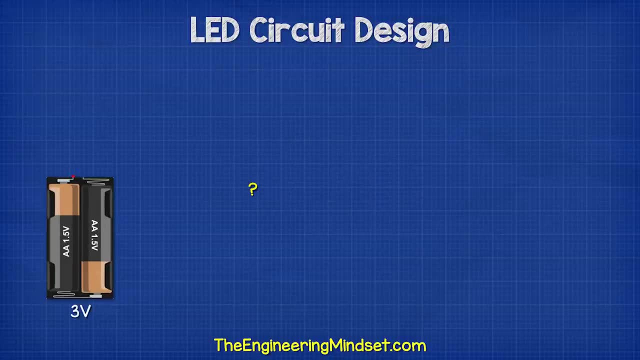 circuits. Let's say we have a circuit that has a voltage drop of 20 milliamps- We can test that with a 3 volt supply- and we want to connect a single red LED. What resistor do we need? Well, we know, this wire is 3 volts and this one is our ground wire, which will be 0 volts. The LED has a voltage. 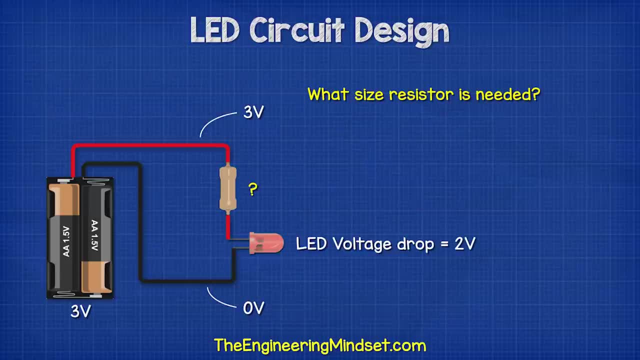 drop of around 2 volts, and so our resistor needs to remove the remaining voltage. So 3 volts subtract 2 volts equals 1 volt. We know the LED needs a current of around 20 milliamps. So 1 volt divided by 0.02 amps equals 50 ohms of resistance. Make sure you convert your milliamps to amps, for 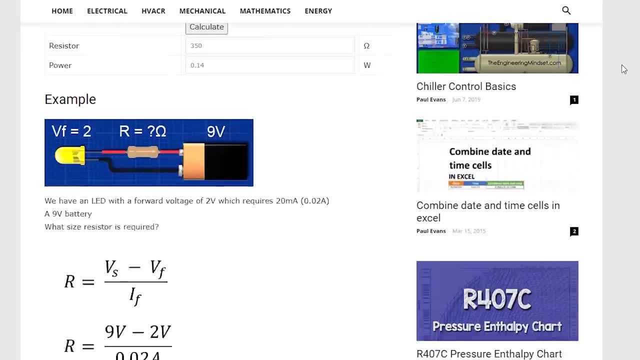 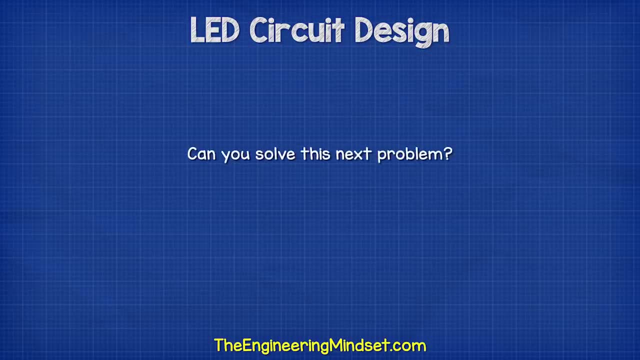 this calculation. To make it easier, we do have a calculator on our website where you can just input your values. I'll leave a link in the video description down below for that. Okay, now you try to solve this one. before I do, Let me know your answers in the comment section down below. 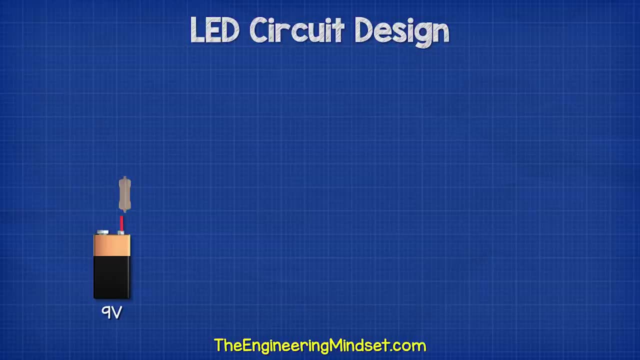 Let's say we have a 9 volt battery and we want to connect a yellow LED which has a voltage drop of 2 volts and requires 20 milliamps of current. So what size resistor is required? Well, we have a 9 volt supply, so subtract 2 volts for the LED and that leaves us. 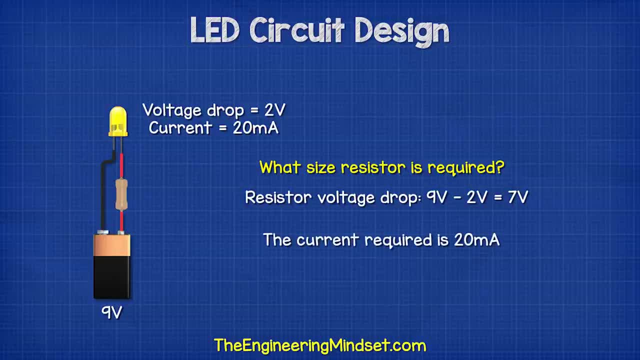 with a 7 volt drop for the resistor. The current is 20 milliamps, so 7 divided by 0.02 amps equals 350 ohms of resistance. Now the problem is that we don't have a 3 volt resistor, so we need to. 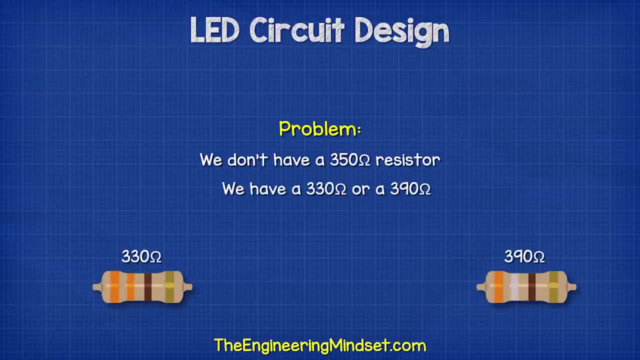 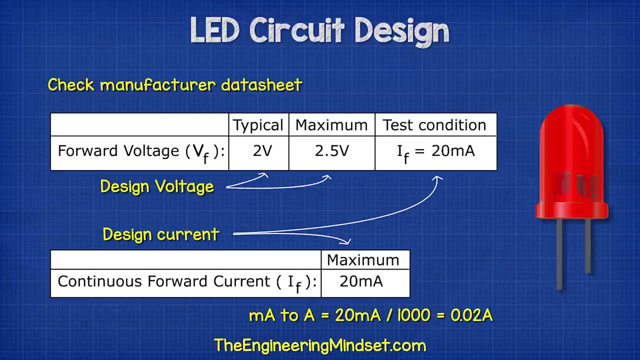 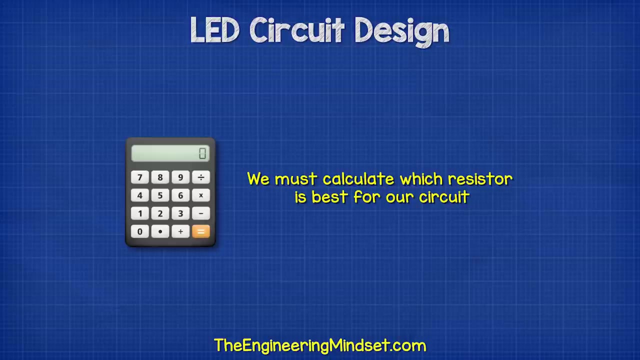 have a 350 ohm resistor. We only have a 330 ohm or a 390 ohm, So which one should we use? As we saw earlier, we need to ensure the current doesn't exceed 20 milliamps, So we will have to calculate which resistor suits us best. To do that, we just divide the 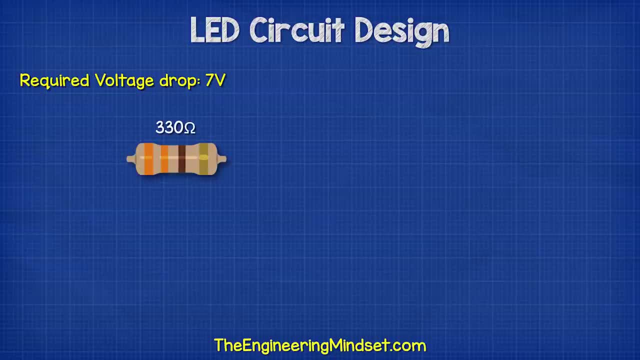 required voltage drop of 7 volts by the resistor value of 330 ohms to get 0.021 amps, And then we'll have to calculate the current value of the resistor value of 0.021 amps. Then if we do the same for the 390 ohm resistor, we will get 0.018 amps. Both of these values are: 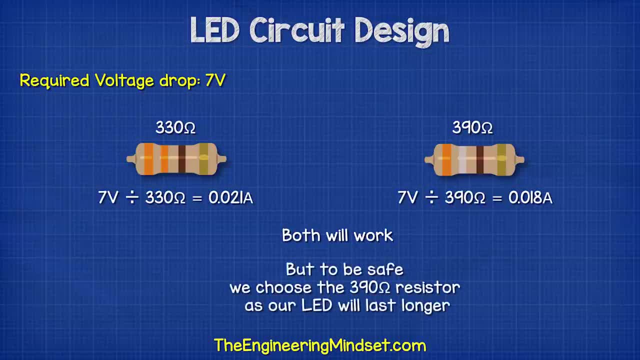 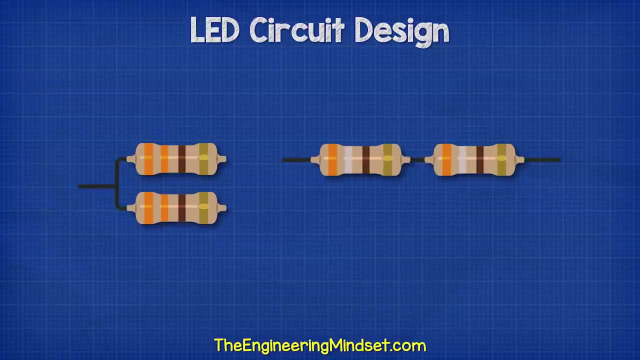 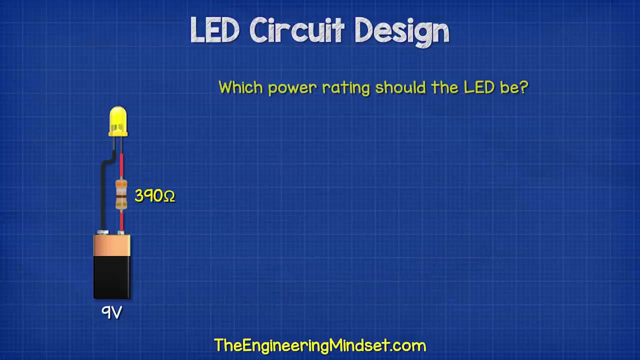 very close and they both will work, But to be safe, we will choose a 390 ohm resistor, as our LED will therefore last longer. We can also combine resistors to get the exact value we need, and I'll explain that a little later in this video. We will also need to choose the resistor power rating. 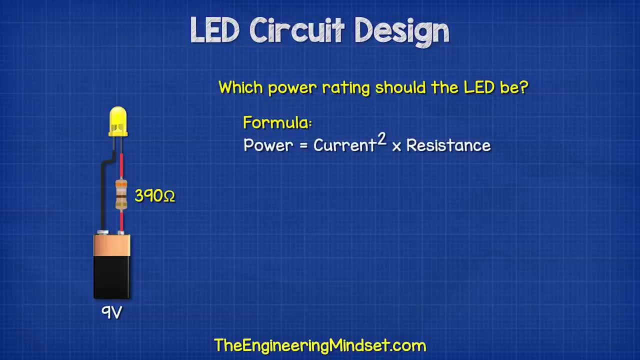 We can calculate this using the formula: power equals current squared multiplied by resistance. So 0.018 amps squared multiplied by 390 ohms gives us 0.126 watts. So a one quarter watt rated resistor will be fine for this circuit. How long will this battery power our circuit for? 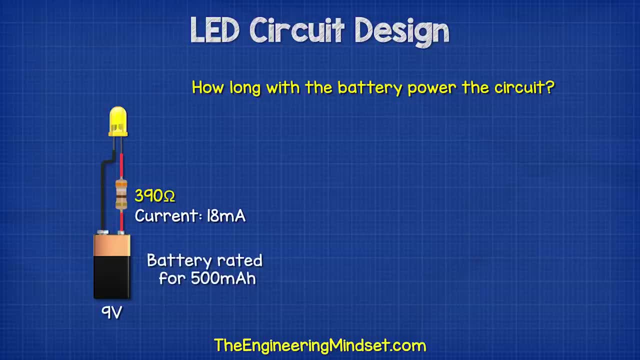 Let's say this battery is rated for a typical 500 milliamp hours. We simply divide this by our total circuit current, which in this case is 18 milliamps. So 500 milliamp hours divided by 18 milliamps will give us around 27 hours, Although this is the very 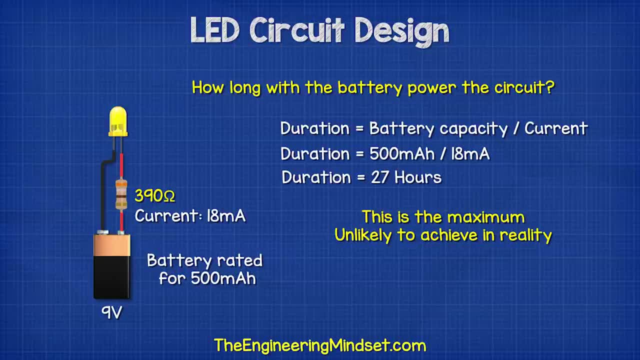 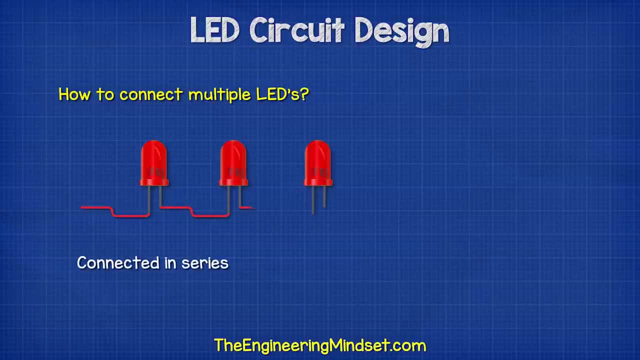 maximum it would power our circuit, for In reality it probably will not achieve this. Okay, so what if we wanted multiple LEDs? One option is to connect them in series. In this design, the voltage drop of each LED will add together, So the total voltage drop in the circuit shouldn't exceed the battery. 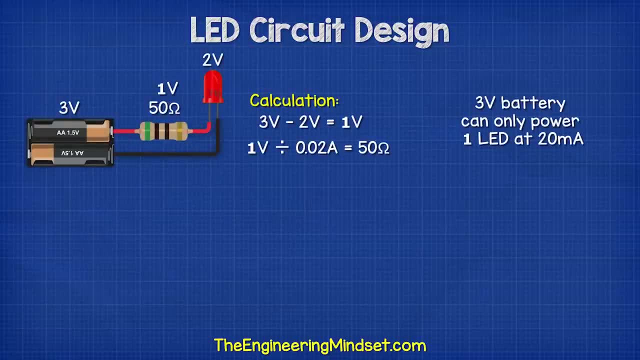 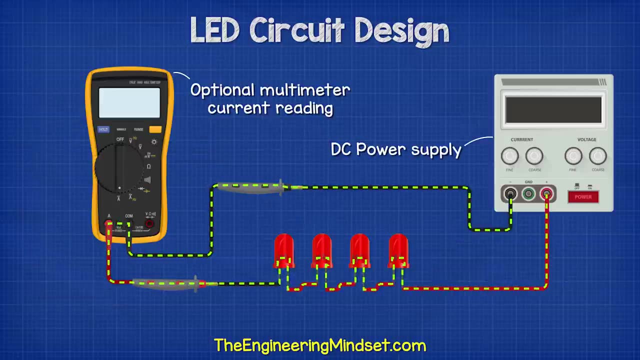 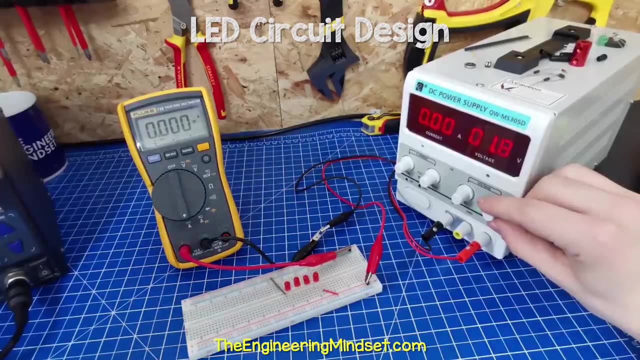 Therefore, a 3 volt battery can only sufficiently power one LED at 20 milliamps and a 9 volt battery can sufficiently power four LEDs. If we connect four LEDs and connect this to our DC bench power supply, we see they will not turn on until their total combined minimum forward voltage is reached. 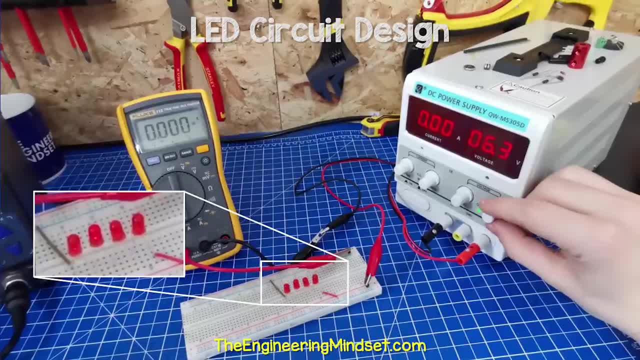 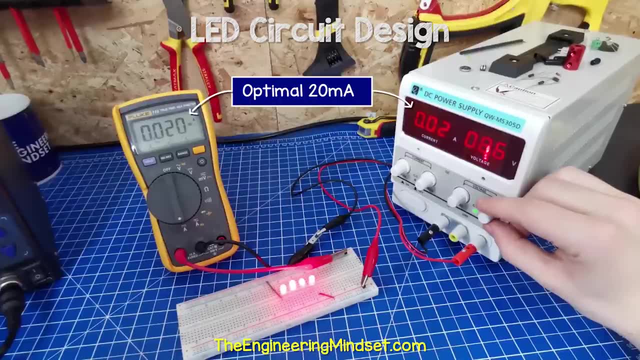 at around 6.3 volts. However, the optimal 20 milliamps of current will not be reached until around 8.6 volts. At 9 volts, the current is around 35 milliamps, which is obviously too high, so we will need a resistor. 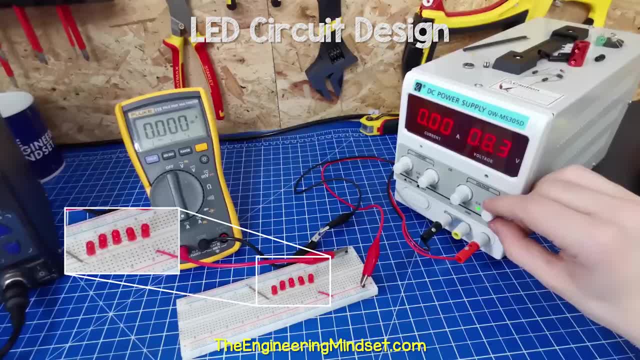 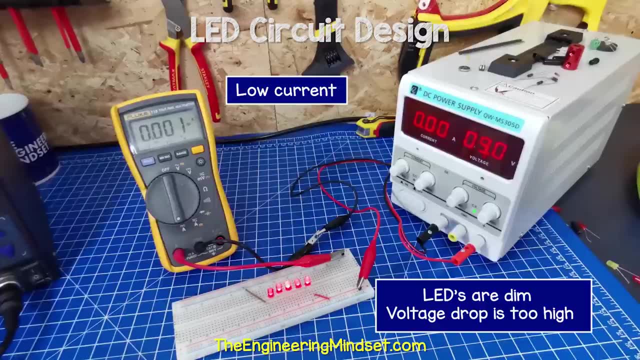 If we connect five LEDs, they won't turn on until around 8.3 volts. At 9 volts they are all on, but the current is very low, so the LEDs are dim. That's because the voltage is low. The voltage isn't enough to fully power the LEDs. 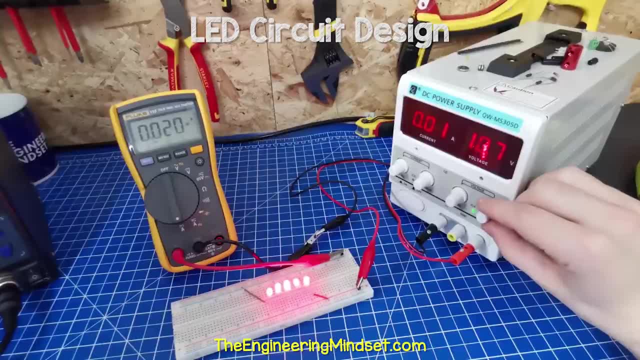 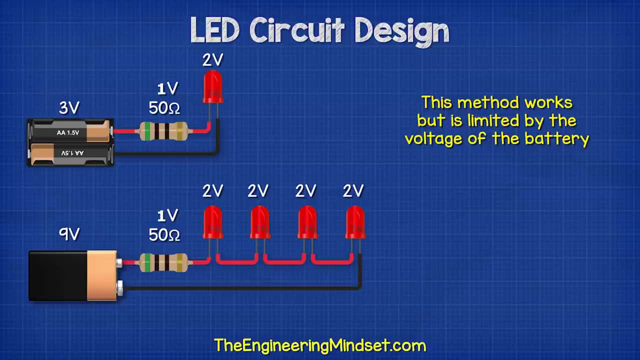 The optimal 20 milliamps isn't reached until 10.7 volts in this example. So we can use this method, but we are limited by the voltage of the battery. What if we want more LEDs? Well, we need to connect them in parallel. 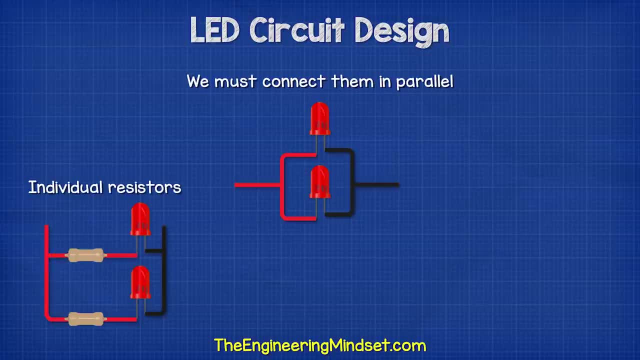 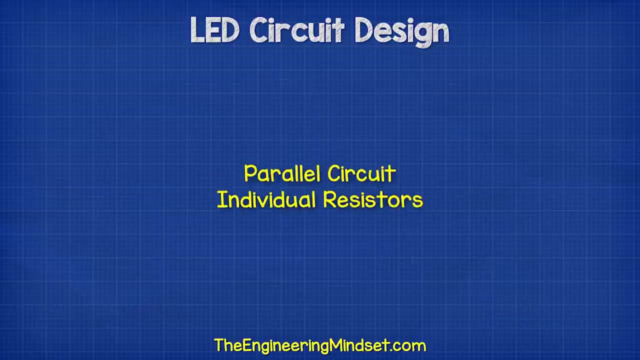 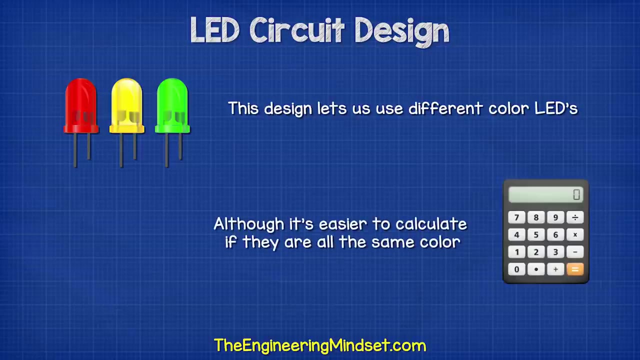 We can either place a resistor on each LED or we can use one resistor to feed all the LEDs. Let's start with the first example. This design lets us use different color LEDs, although it's easier to calculate if they are all the same color. 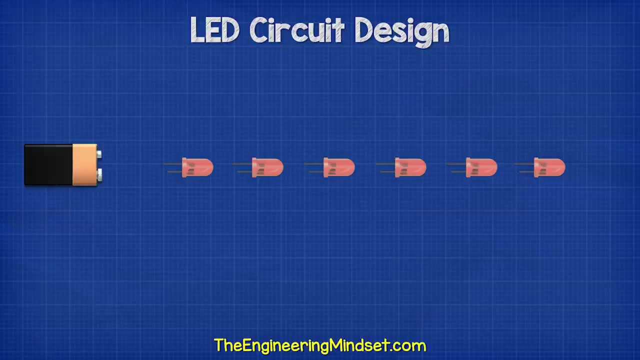 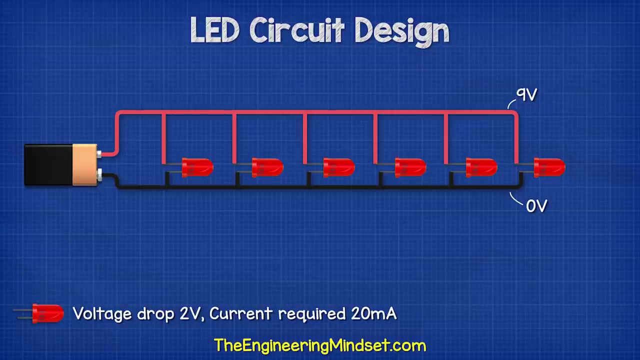 Let's say we want to connect six LEDs to this 9 volt battery. Each LED has a voltage drop of 2 volts and requires 20 milliamps. This entire rail is 9 volts and this entire rail is zero volts, So each LED will get 9 volts across it. 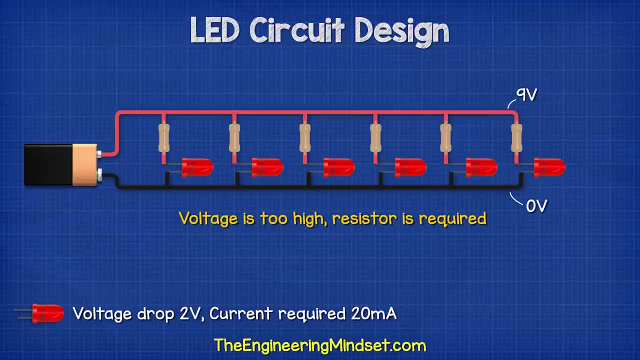 That's obviously a lot, So we will need to place a resistor against each LED. So we have 9 volts. subtract 2 volts for the LED, which leaves us with 7 volts, So we need to drop 7 volts on each branch. 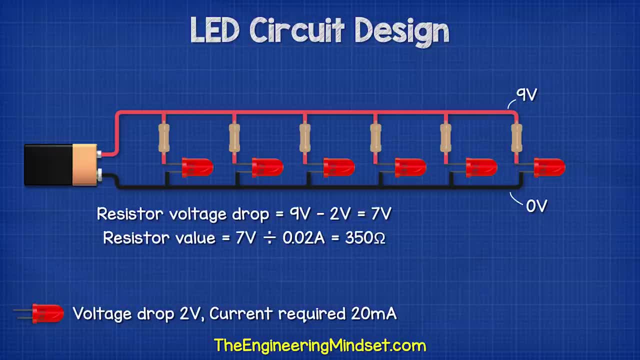 We calculate the resistor value by 7 volts divided by 0.02 amps, which equals 350 ohms, And then we find the power rating, So 0.02 amps squared multiplied by 30. 350 ohms gives us 0.14 watts, so a 1.25 watt resistor will be used. 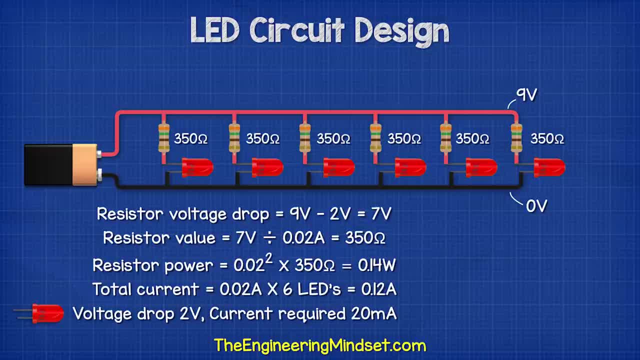 Then we need to add up all the currents in each branch, So 0.02 amps multiplied by 6 LEDs gives us 0.12 amps. A 9 volt battery has a capacity of around 500 milliamp hours And our circuit is using 120 milliamps. 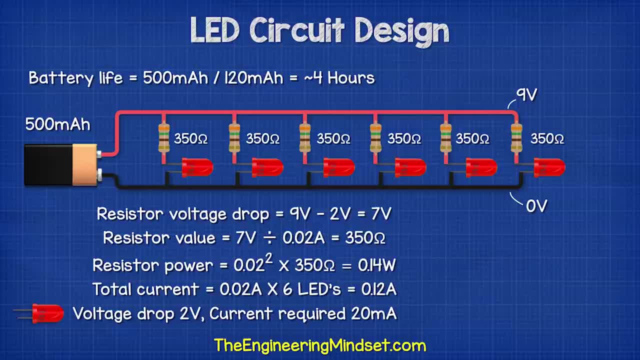 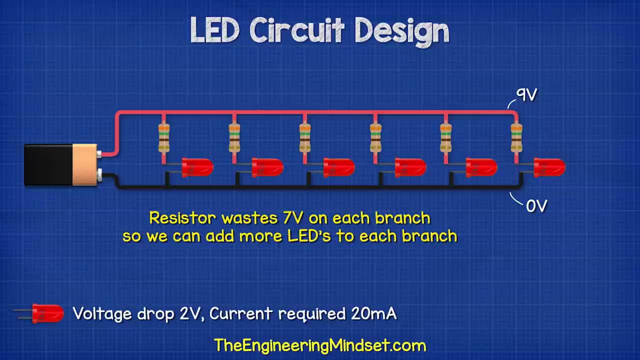 So 500 divided by 100 milliamps, That gives us around 4 hours of run time. We can see that there is still enough voltage on each branch to connect more LEDs. Let's say we place 3 LEDs on each branch. 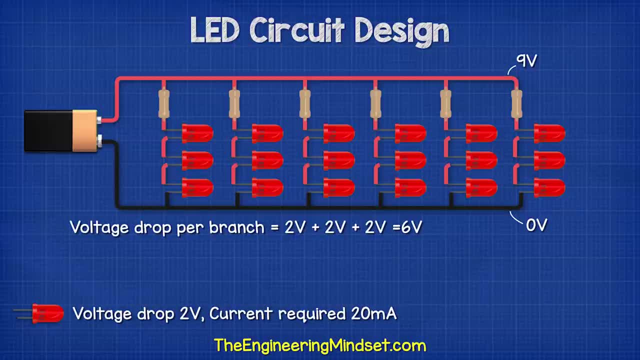 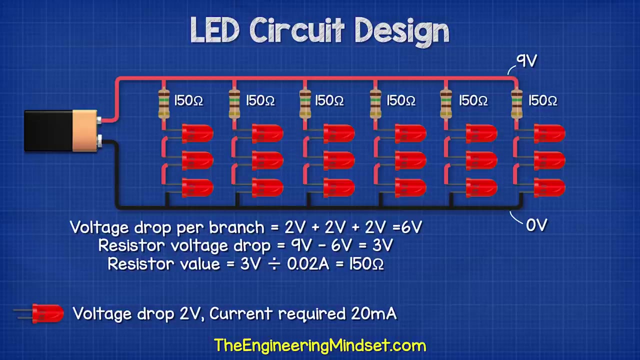 So each branch has a reduction of 6 volts. Therefore, 9 volts subtract 6 volts equals a 3 volt drop by the resistor. So 3 volts divided by 0.02 amps gives us 150 ohms. Notice, the total current in each branch didn't increase. 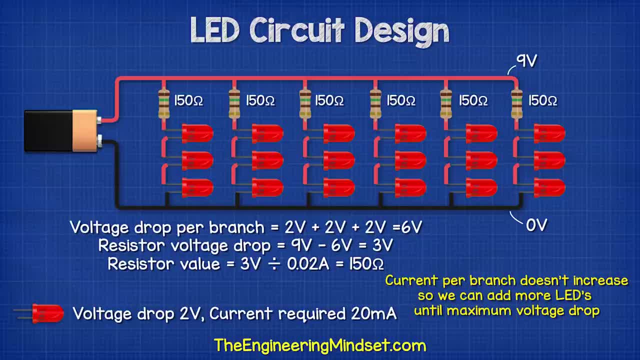 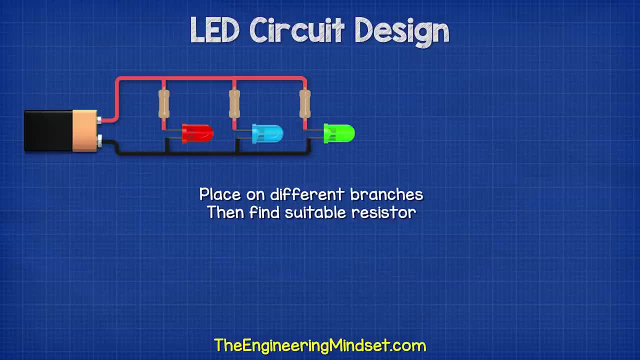 So we can add more LEDs until the maximum voltage is reached. If we want to use different color LEDs, then we place the different LEDs on the different branches and we find the suitable resistor. For example, we might have a red, blue and green LED. 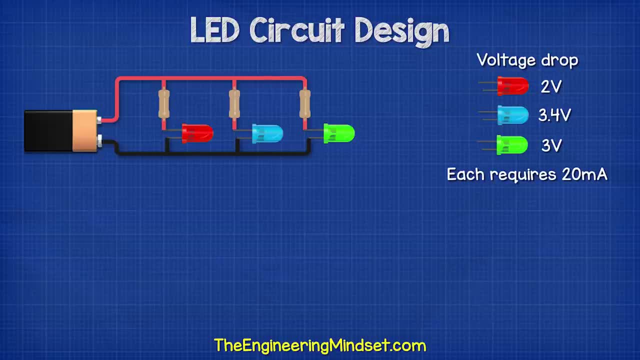 Each LED has the same current requirement of 20 milliamps, but the red LED has a voltage drop of 2 volts, The blue has 3.4 volts and the green has 3 volts. The resistor for the red LED is therefore 9 volts subtract 2 volts, which gives us 7 volts. 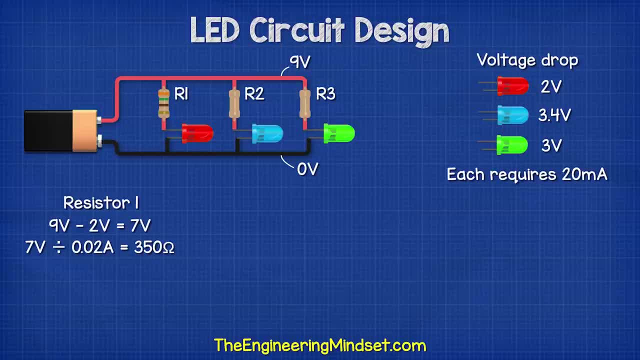 7 volts divided by 0.02 amps will lead us to a 350 ohm resistor. The blue LED is 9 volts subtract 3.4 volts, which leaves us with 5.6 volts, So 5.6 volts divided by the current of 0.02 amps. 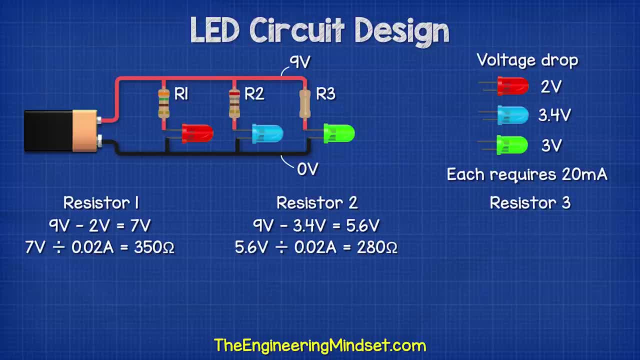 leaves us with a 280 ohm resistor, And the green LED will be 9 volts subtract 3 volts, which leaves us with 6 volts. 6 volts divided by the current gives us a 300 ohm resistor. The total current is therefore 60 milliamps. 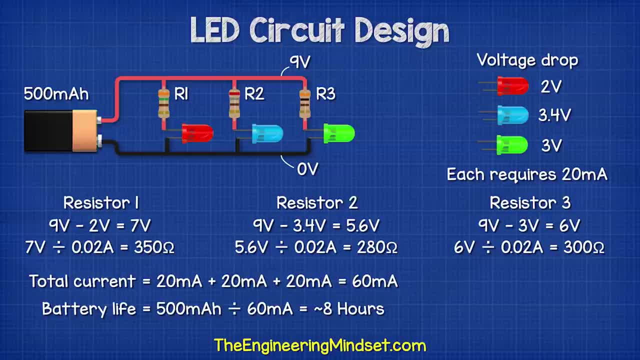 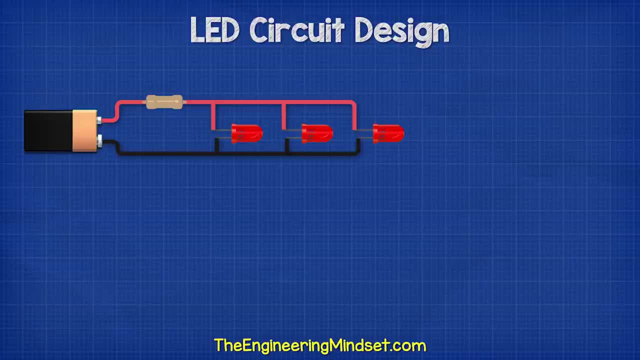 So the battery will last around 8 hours. The other way we can connect LEDs is by connecting them in parallel and then using a single resistor to limit the total current. For this design, you should only use the same color or the same rating LEDs. We'll see why that is shortly in this video. 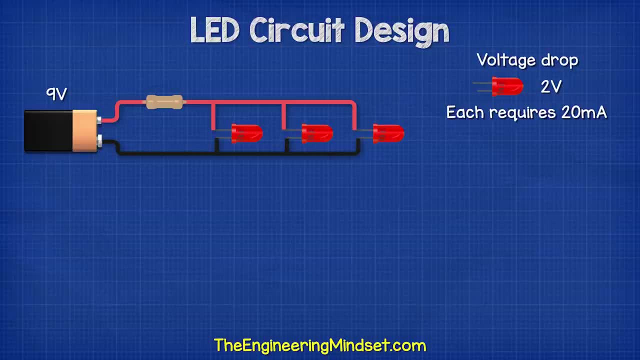 Let's say we have a 9 volt battery and 3 red LEDs, all with the same voltage drop of around 2 volts, and they each require 20 milliamps of current. So we just add the currents together to get 60 milliamps and that current has to flow through this one resistor. 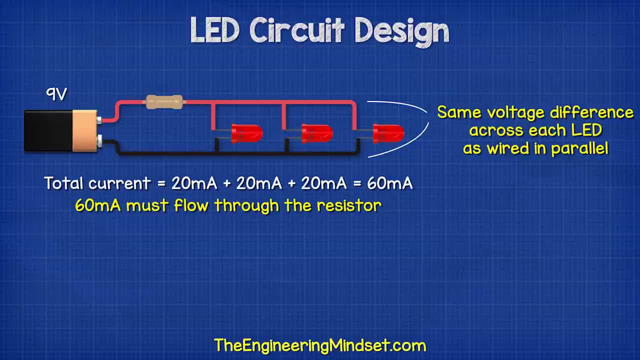 So we just add the currents together to get 60 milliamps, and that current has to flow through this one resistor. Now, as they are connected in parallel, they will all have the same voltage difference across them. Therefore we calculate the resistor by 9 volts. subtract just 2 volts equals 7 volts. 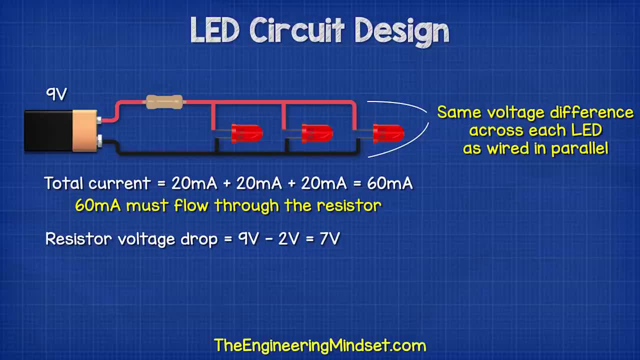 Then, as all the current is flowing through this one resistor, we will need to divide the 7 volts by the 60 milliamps, and that will give us a 116 ohm resistor. The power calculation comes out at 0.49 watts, so a half watt resistor will. 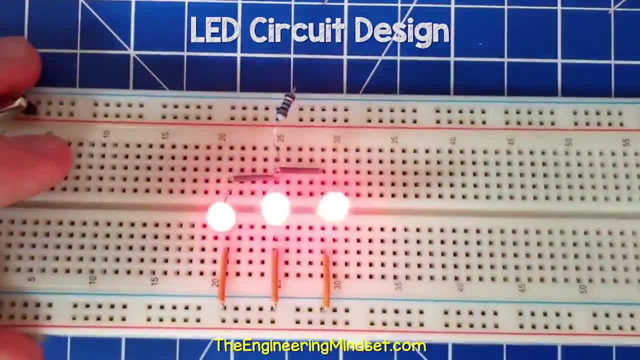 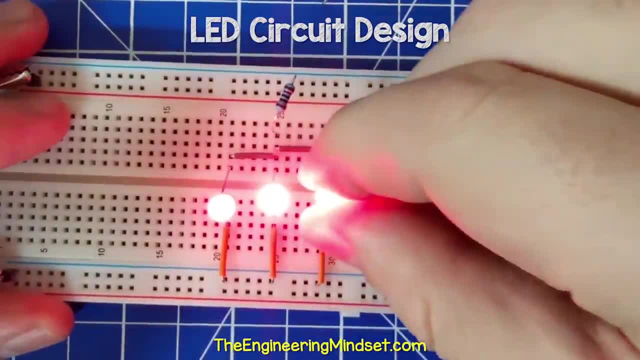 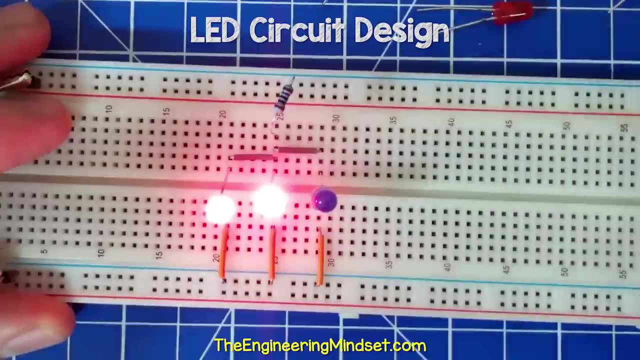 be used. The reason we need to use the same rating LEDs is because the voltage difference across here is just 2 volts. So if we use the same rating LEDs they will all illuminate. But if we place a blue LED in the circuit, this requires a higher voltage. 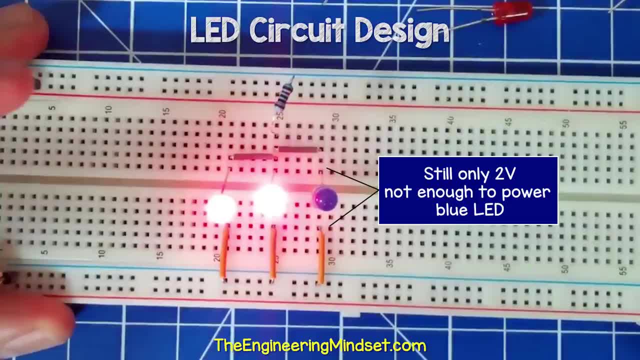 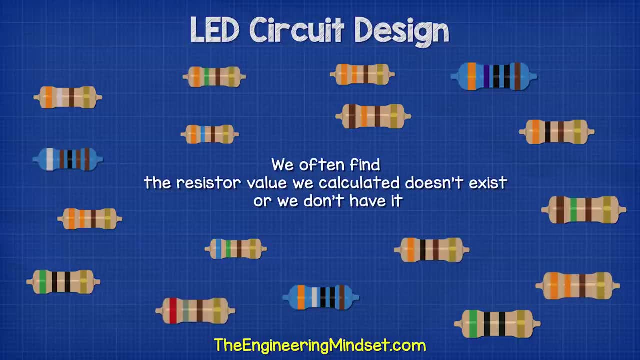 which it will not be able to get. So this LED will not turn on Now. when we deal with these circuits, we often find that the voltage difference between these circuits is very small. We often find that the resistor value we have calculated doesn't exist, or we simply don't have it in stock. 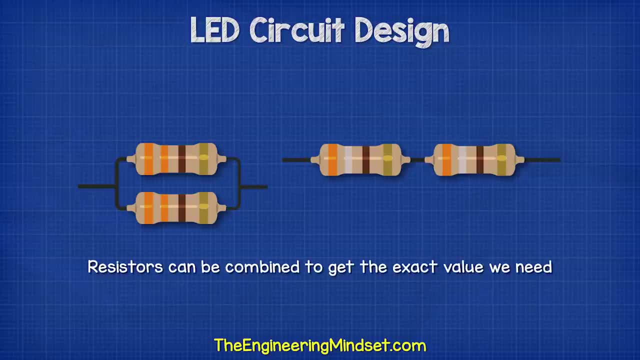 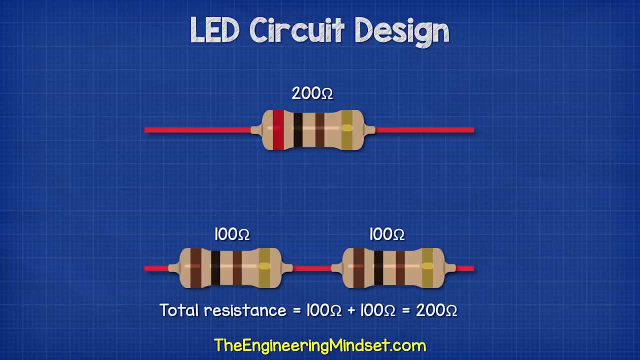 So we can combine resistors to get the value we need. For example, if we wanted a 200 ohm resistor, we could place two 100 ohm resistors in series. or we could place two 50 ohm resistors and a 100 ohm resistor. 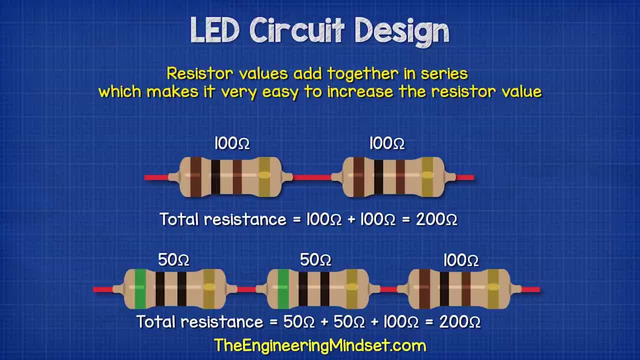 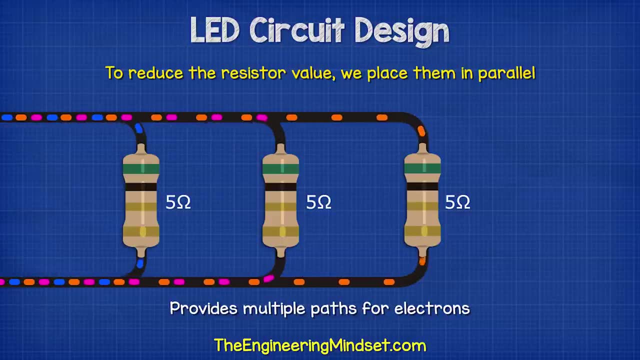 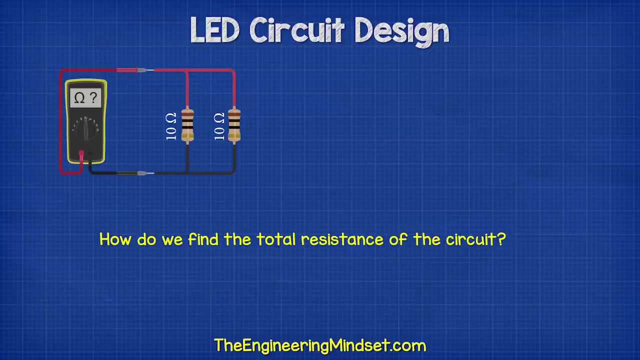 The resistor values will just add together in series, which makes it very easy to increase the resistor value. To reduce the resistor value we simply place them in parallel. Then we do some maths to find the equivalent resistance. Let's say we have two 10 ohm resistors. We can calculate that using this formula. 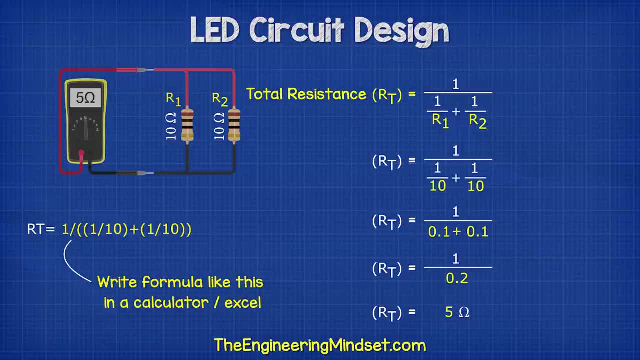 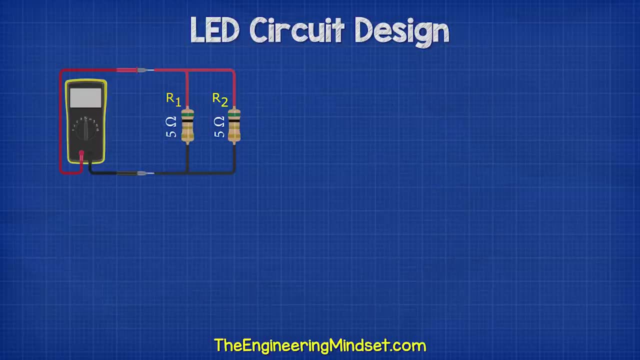 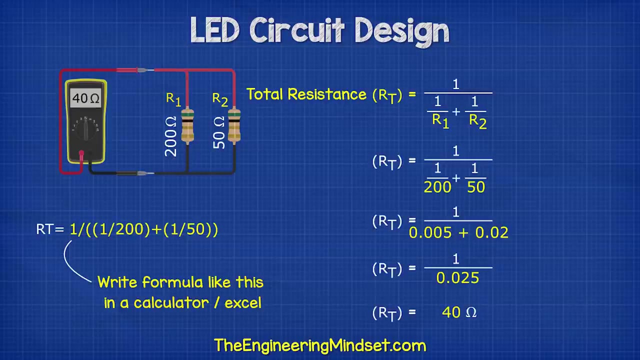 This is much easier than it looks. We just enter this into our calculator and we see it gives us 5 ohms of equivalent resistance. So two 5 ohm resistors will give us 2.5 ohms of total resistance. A 200 ohm and a 50 ohm resistor will give us 40 ohms of resistance. 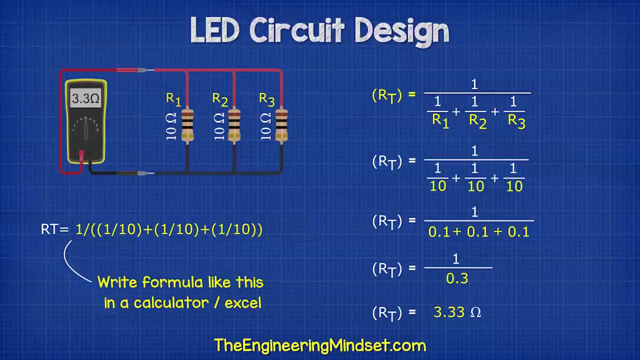 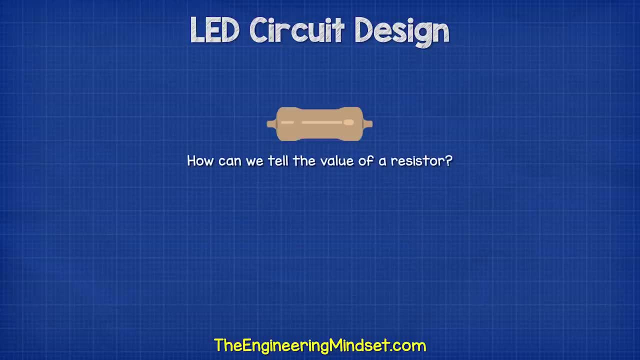 And three 10 ohm resistors would give us 3.33 ohms of resistance. How can we tell the value of a resistor? Well, these colored stripes on the body will tell us the value, but we will need to look it up on a chart. We can get four or five band resistors typically. 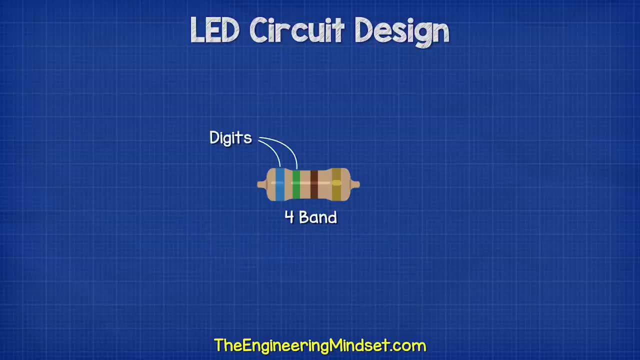 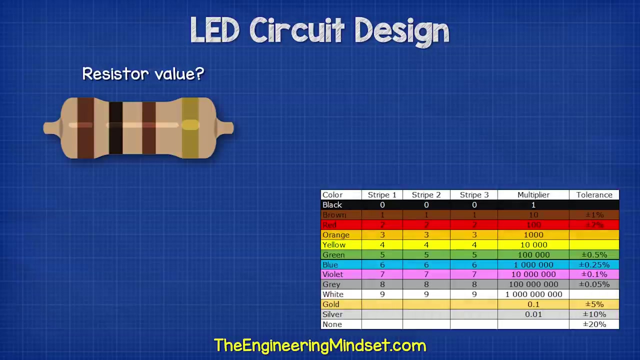 So let's look at some examples of these With the four stripe type. the first two stripes are the digits which we combine, The third stripe is the multiplier and the fourth stripe is the tolerance. For example, this four band resistor is brown, black, brown and gold.